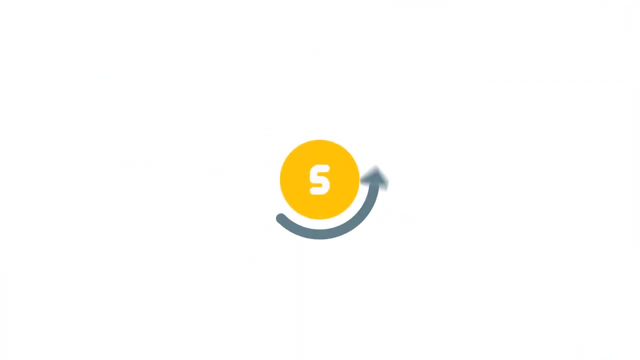 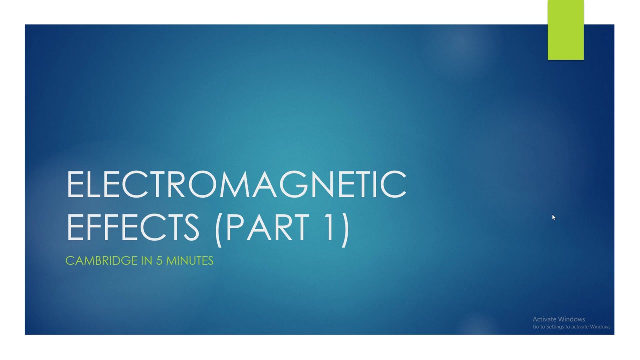 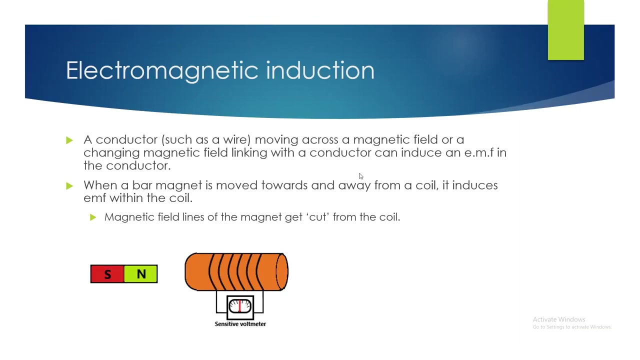 Hey guys, welcome to another IGCSE physics revision video. Today we're going to be going through the first part of the topic of electromagnetic effects. So an electromagnetic induction is the phenomenon where a conductor, such as a wire, which moves across a magnetic 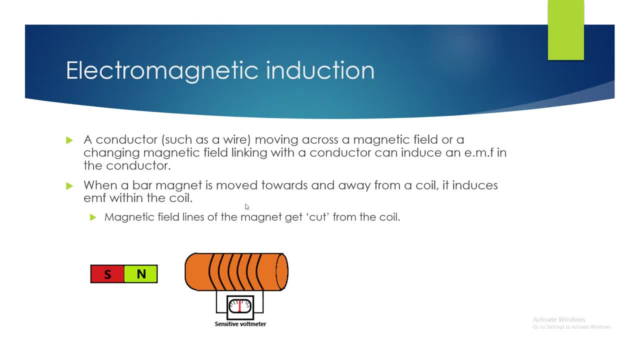 field or in a setting where a changing magnetic field is within the vicinity of a conductor, it will induce an EMF or a voltage across that conductor. So, for example, when a bar magnet is moved towards and away from the coil, it will induce an EMF within the coil. Why? Because the 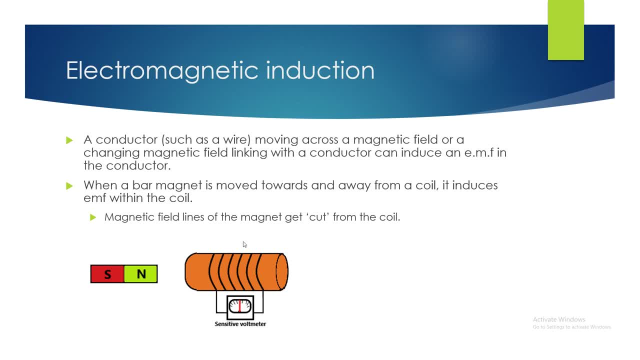 magnetic field lines of the bar magnet become cut from the coil as the magnet is moved in and out, And so therefore, when the EMF is in the vicinity of a conductor, it will induce an EMF or a voltage across that conductor, So an EMF is produced. you will get a brief reading on the sensitive 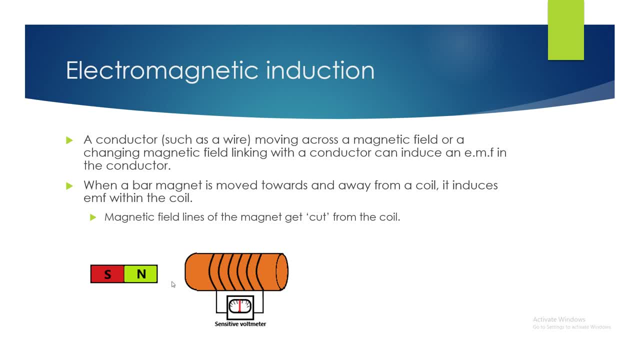 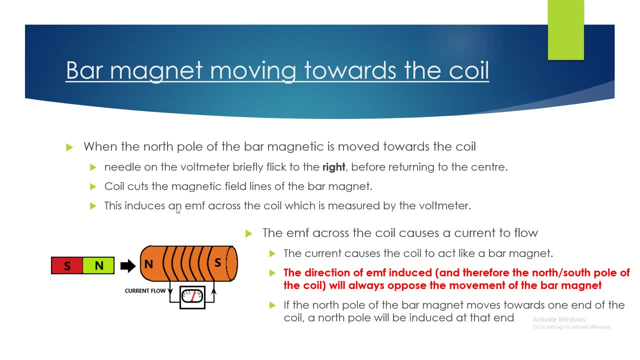 voltmeter and the direction of that depends on how we move the bar magnet, which we will look at now. So the bar magnet moving towards the coil. Okay, so when the north pole of the bar magnet is moved towards the coil, like in this diagram shown, the needle on the voltmeter will briefly flick to the 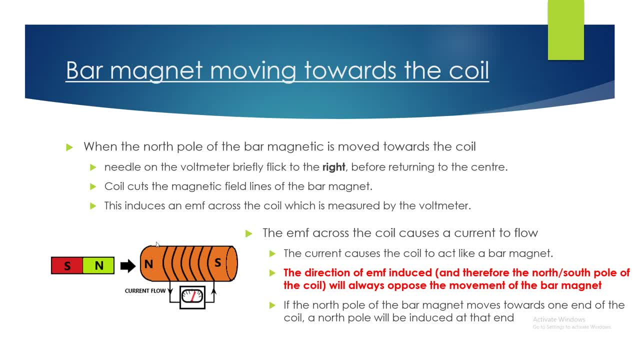 right before returning back to the center, And so this is because the coil cuts the magnetic field and the current is flowing in a particular direction. So the bar magnet is the magnet that induces an EMF across the coil, which is then perceived by the voltmeter, And so the EMF that 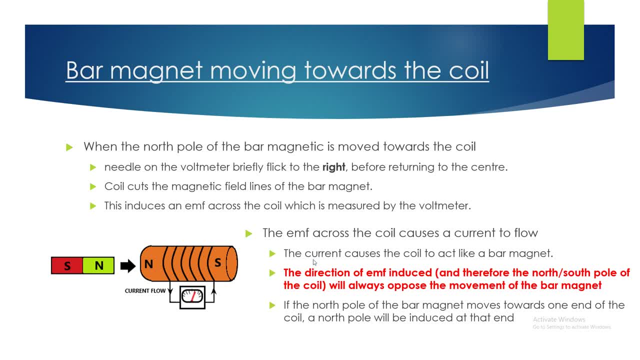 gets induced across the coil causes a current to flow in a particular direction. Now, when you have a current flowing within the coil, then you will actually allow that coil to become a temporary magnet and behave like a bar magnet. And with any sort of magnets you're going to have a north and 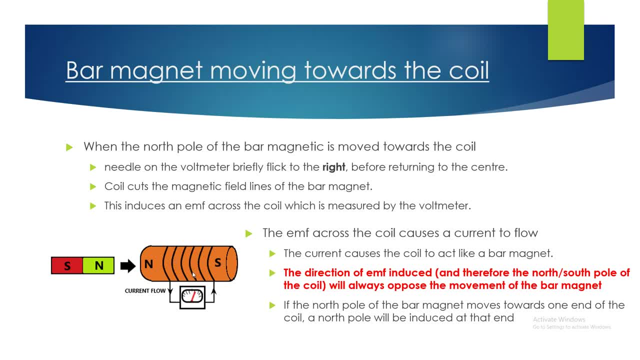 south pole And the EMF will then flow in a particular direction. So when you have a current that gets Induced, pole on the coil is going to be always in a way that will oppose the motion of the bar magnets. So, for example, here we're moving the north pole closer to the coil And so 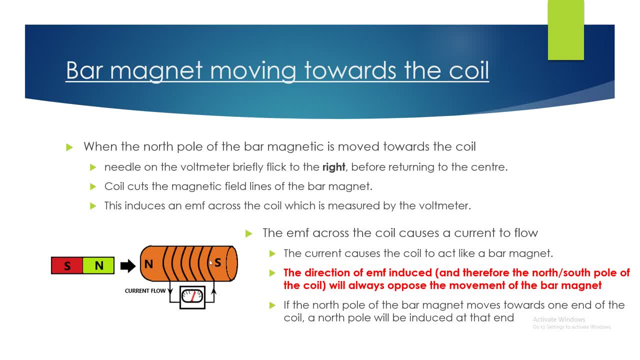 therefore the direction of EMF and the direction of current, causing a north and south pole to form on the coil. the poles will be positioned to oppose the movement of the bar magnet. So therefore, in this case, because EMF is indefinite and current isáspant, the bar magnet is usually subject to. 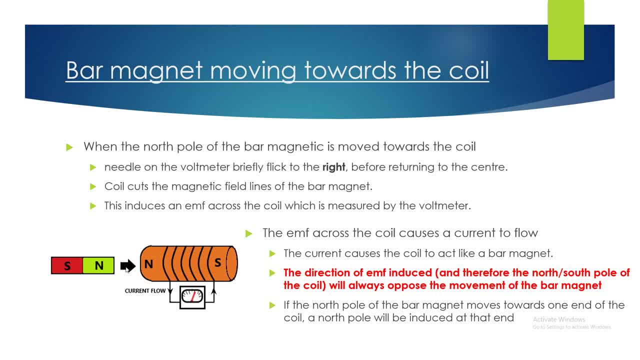 motion of the bar magnet. But you can actually see that this is because the dressing coil is light. poles repel each other and it wants to push the bar magnet away. you're going to get a north pole that is formed or induced closest to the north pole of the bar magnet, which is moving. 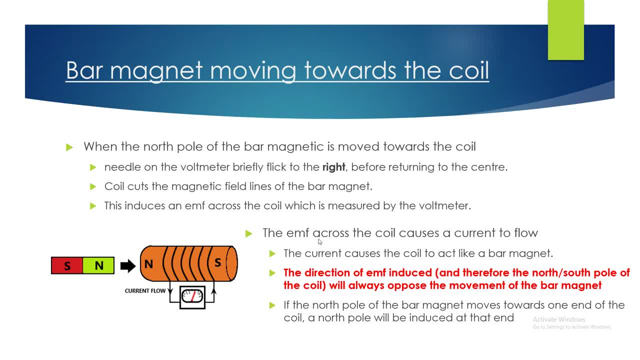 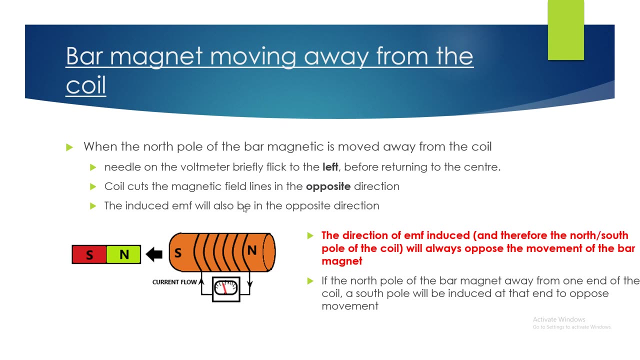 towards the coil. okay, so you always just need to understand that the poles that will be formed in the coil will try to oppose the movement of the bar magnet. so what happens when we do the opposite? what happens when we move the bar magnet away from the coil? well, when the north pole of the 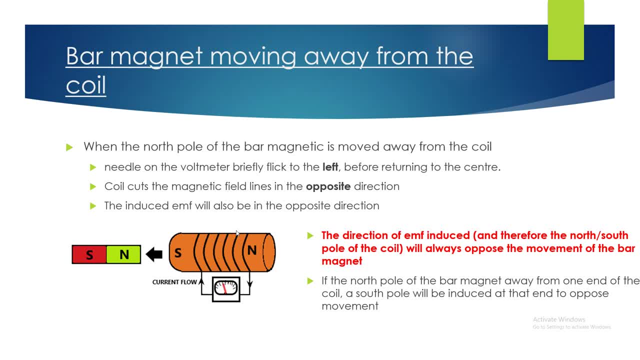 bar magnet is moved away from the coil, then the needle on the voltmeter will briefly flick to the left. recall the last time when we pushed the magnet towards the coil and moved to the right. so this is going in the opposite direction this time. why the coil again cuts the magnetic fields. 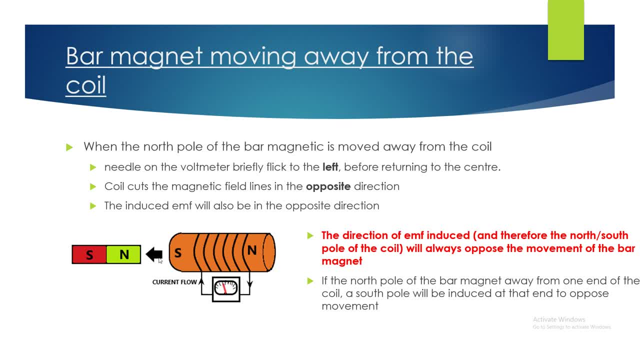 but this time in the complete opposite direction, as the bar magnet is moving away from the coil, so the induced emf will also be in the opposite direction and again, as we've discussed before, the poles that are that are induced in the coil will always try to oppose the movement of the bar magnet. this time it's going. 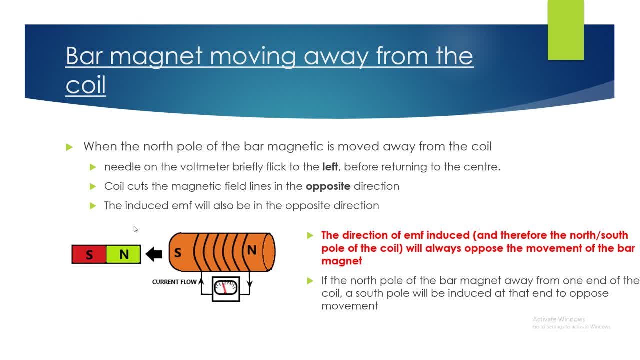 away from the coil and it wants to keep it close to it, so it's going to try to pull it in. so again, the poles- opposite poles- will attract each other. so therefore, closest to the north pole on the left hand end of the coil, you're going to get an induction of the south pole. 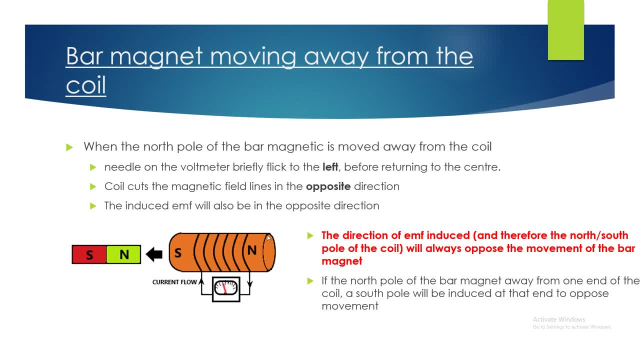 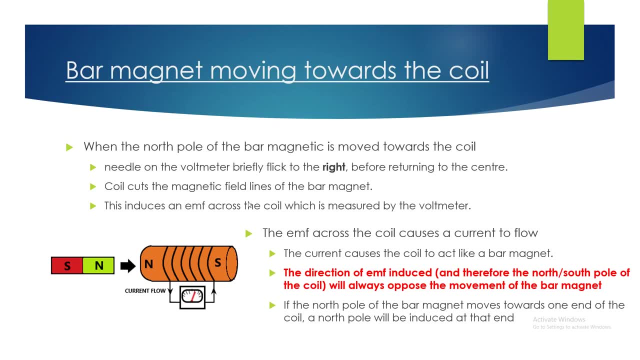 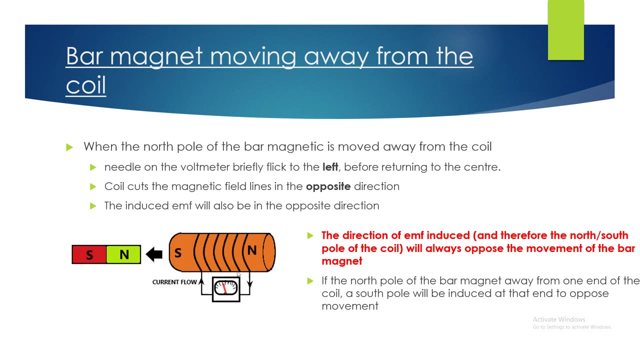 and so if you were to really try to dig deeper and figure out the direction of current, because, as you can see here, uh, this first time when the magnet was moving towards the coil, the current flow was in this particular direction, and the second time we did it, the current flow was going. 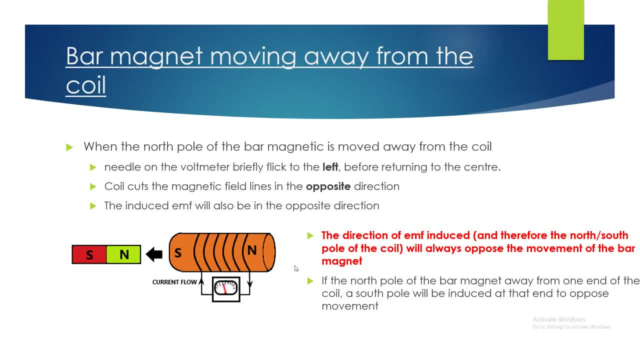 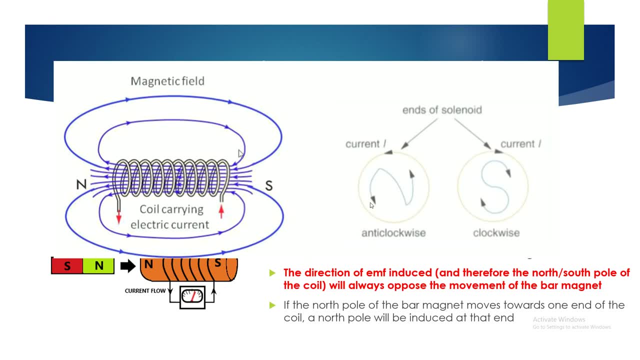 in the opposite direction. and if you want to figure out the actual direction of current, then all you need to do is back trace. so remember when we took a look at the direction of current in a solenoid and how, depending on that direction, and it induces a certain pole. well, if we have a 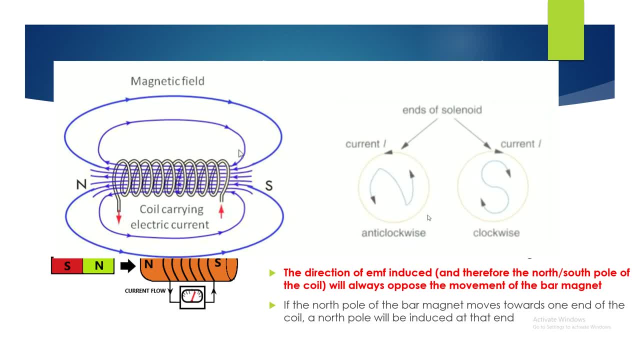 north pole here, like we do, then you want to know that the current flow will be anti-clockwise, as opposed to, if you've got a south pole, then you know that the current flow is going to be clockwise. so you're just back tracing from what you already know. and uh, if you aren't, 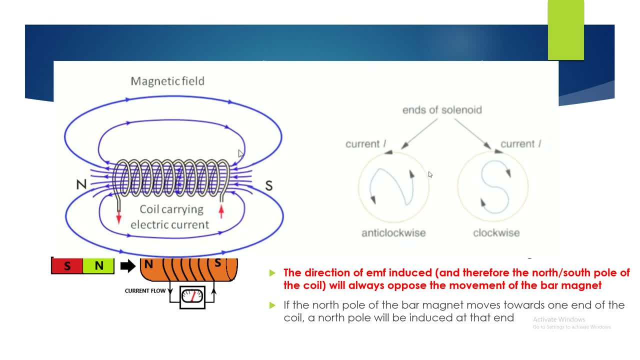 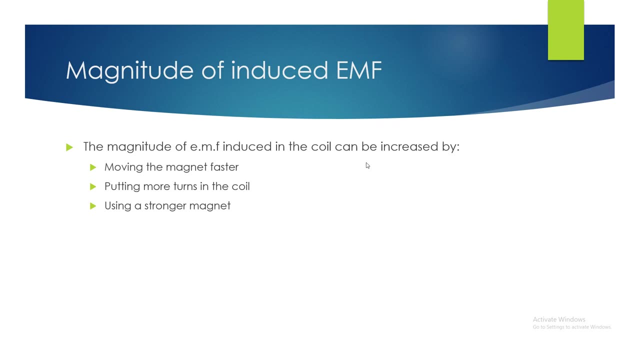 familiar with this, then check out my previous videos, because we've covered um how the current within a solenoid will induce a certain magnetic pole within. Okay, so the magnitude of the induced EMF can be increased by three things. One: moving the 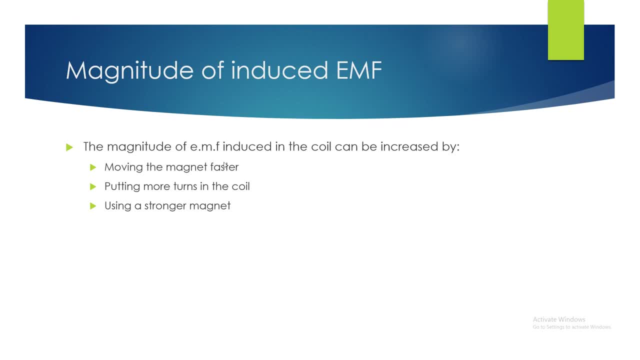 magnet closer, or sorry, faster. Two, putting more turns in the coil that you use. And number three, using a stronger magnet. So now that we know the fundamentals of the phenomenon of electromagnetic conduction, we're going to use that to create AC current. So there's two types of current: The 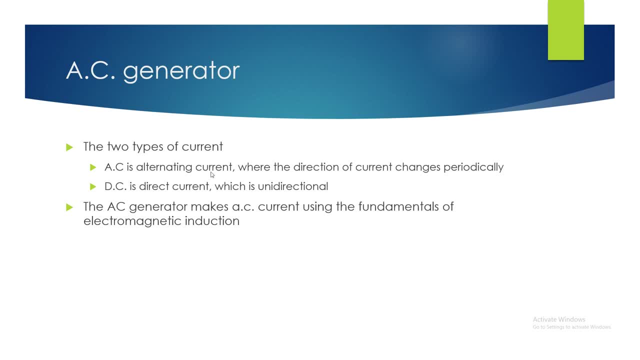 first one is AC current, which is alternating current. This is when the direction of current changes periodically, whereas DC current is a form of direct current which is unidirectional. It doesn't change in direction at all. So the AC generator makes AC current using the fundamentals. 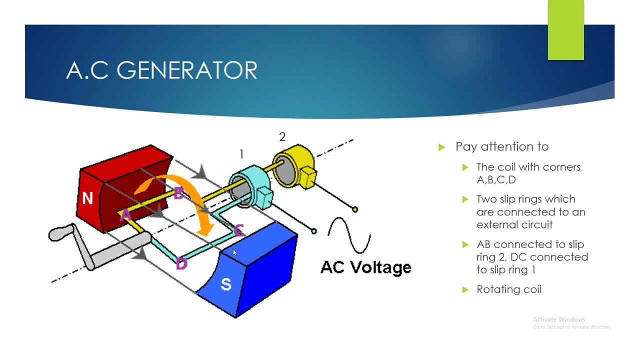 of what we talked about before. It is a little bit complex, so let's have a look at this. It's made up of a north and south pole of a magnet, So you get the field lines of the magnet going from the north to south Within the two magnetic fields. you're going to have a coil. 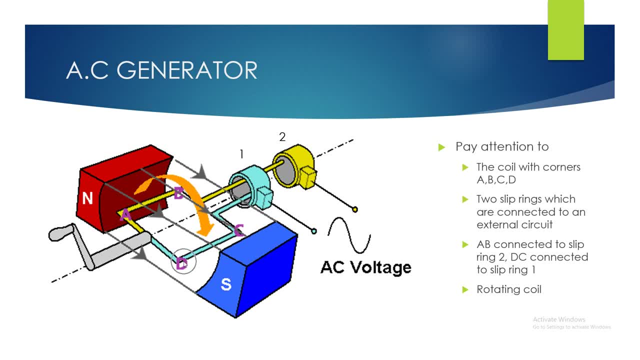 that I've labeled A, B, C and D at each corner, And so this coil is going to be rotating around and around and around. And so the side AB, which is the yellow side that I've labeled here, is connected to slip ring 2.. 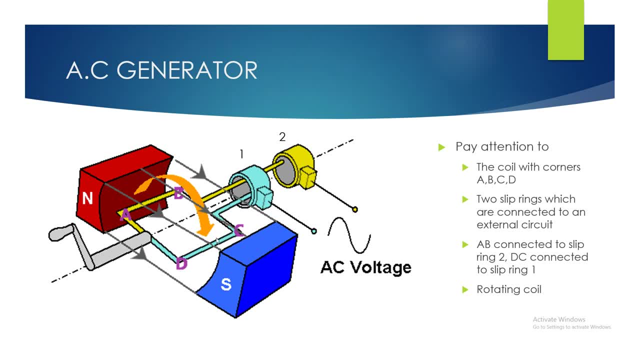 And the side C and D is the blue side, which is connected to the first slip ring, And each of these slip rings are connected to an external circuit. Of course, as the coil rotates around and around, this is going to start to generate alternating current within the external circuit that it is. 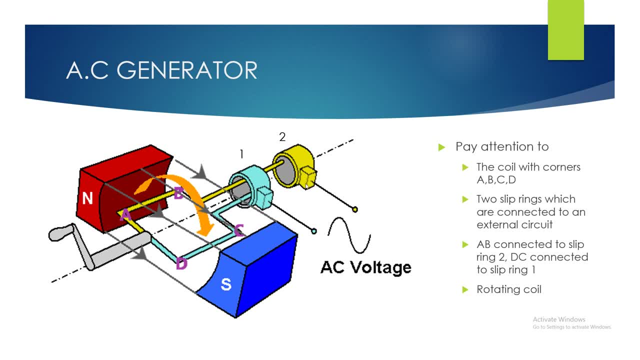 connected to, And we'll demonstrate how that happens. So, first things first. as the coil moves around, rotates, you know, in this case clockwise- you're going to see that the coil will cut the magnetic field lines along the way. And as it cuts the magnetic field lines, this is going. 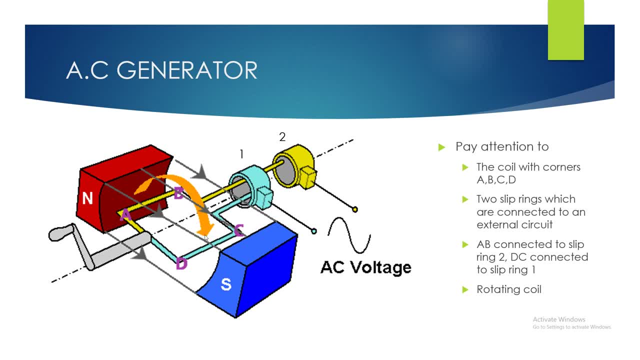 to generate some sort of electromotive force, or EMF, within the coil and it's going to generate the current, And how exactly it produces alternating current is what we will discuss in a bit more detail. So, as we've discussed before, the magnetic field lines, 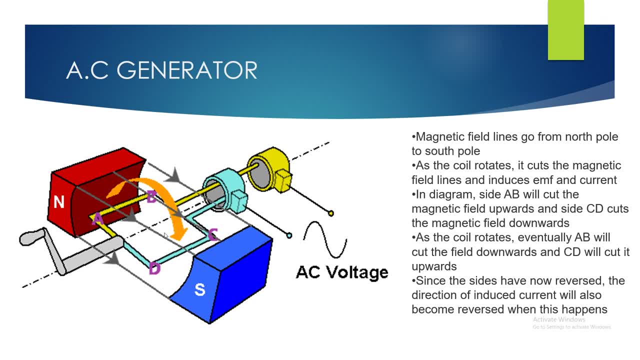 we'll go from north to south pole And you can see that as the coil rotates, the side AB will actually cut the magnetic field lines upwards, whereas CD will cut the magnetic field lines downwards in this particular example. Now, eventually, as the coil rotates, you'll end up having side A and B on this. 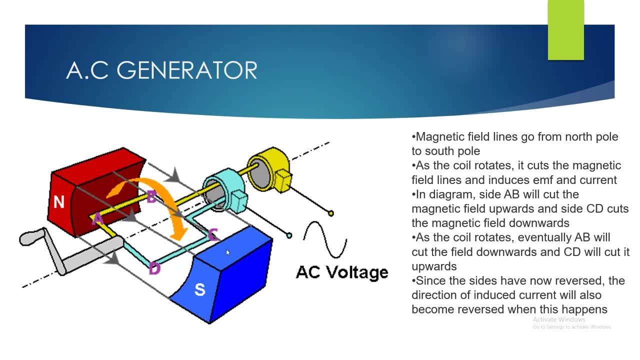 right-hand side and C and D on the left-hand side as it rotates further. Now, when side AB hits this right-hand side here, then it's going to start to cut the coil- sorry, to cut the magnetic field lines downwards this time. 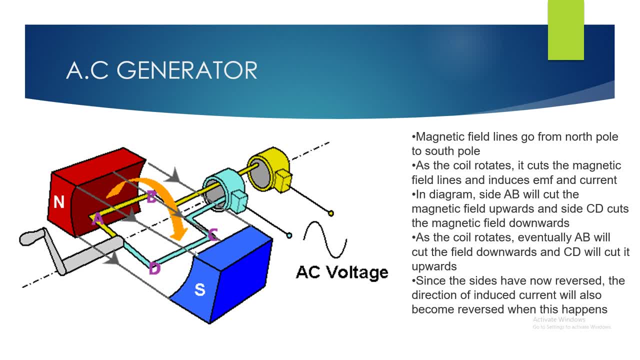 It was cutting it upwards on the left-hand side, but it'll start to cut it downwards on the right-hand side and vice versa. for this side here, D and C, When it reaches the opposite end, it's going to cut the field lines upwards. So each time this reverses itself, you're going to get an electromotive. 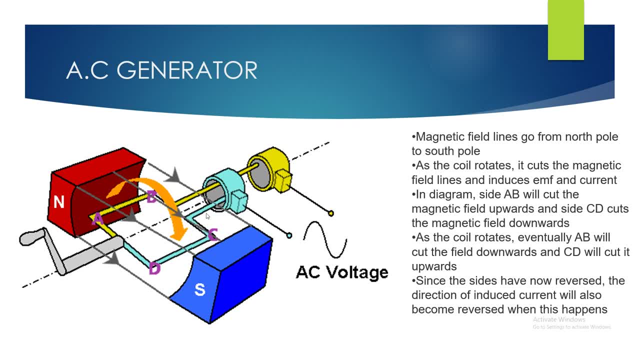 force that is going to produce current in an opposite direction. Okay, so you get EMF produced in the opposite direction when the coil cuts the field lines downwards. So every time AB switches over or D and C switches over inside, you'll get a reversal of the direction of current. 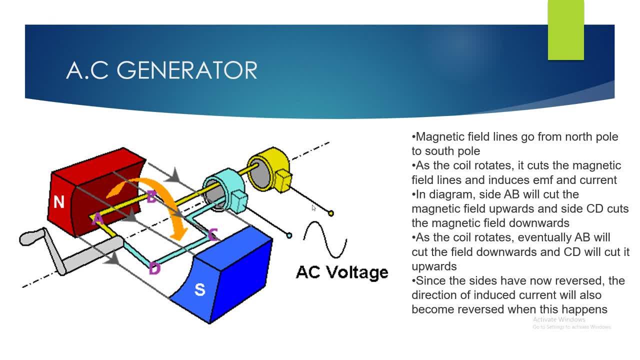 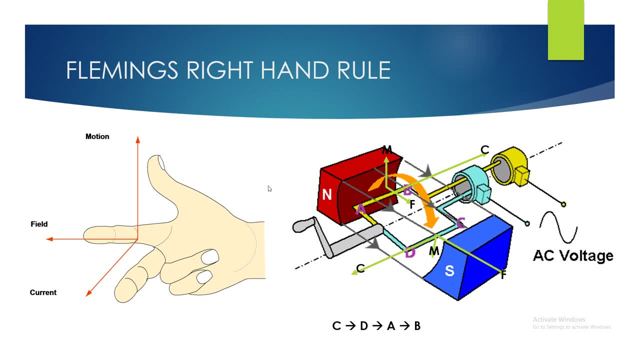 I know that might be a little bit confusing at the moment, but we'll get to that in just a moment. going to take a deeper look at this using the fleming's right hand rule. so the fleming's right hand rule is basically use your right arm and white right hand to align your fingers like this. 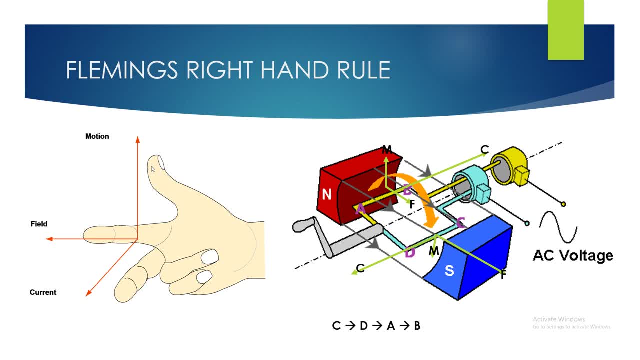 the motion is, of course, the motion of the coil or the side of the coil that is moving in a particular direction. you've got the field, which is the direction of the magnetic field lines, and you've got the direction of current. of course, in this particular scenario, we know the motion and we know. 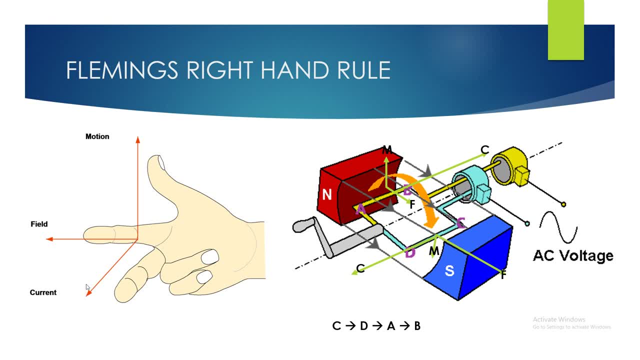 the fields. and this last bit: your middle finger is going to give you the direction of the current. so align your right hand, using this rule, with side a and b. you'll instantly notice that your middle finger will point in this direction here, suggesting that current is flowing in that particular. 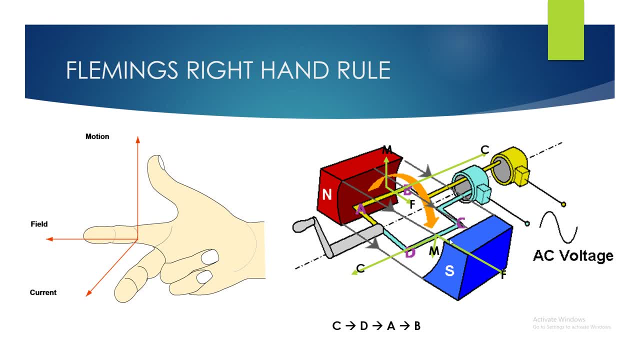 direction. if you were to do the same for the side d and c of the coil, you'll actually get the current going, uh, in this direction. so you know that current is going to be induced in the direction of c to d, to a to b. okay, so that's the direction of current that you'll get in this particular 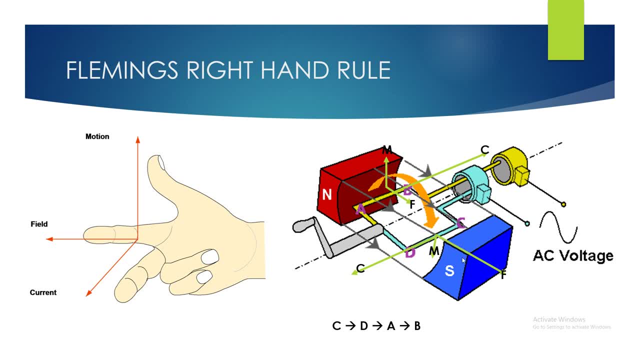 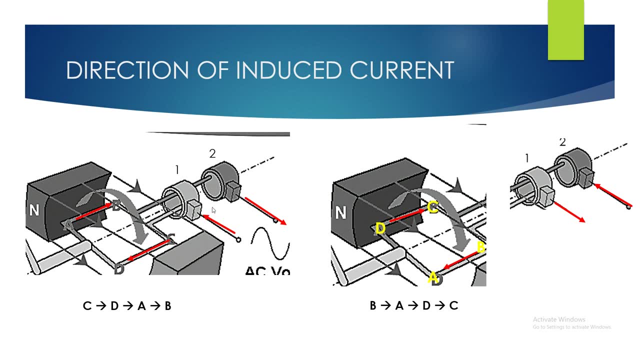 instance, with a and b being on the left hand side and c and d being on the right hand side of the bottom. okay, so this is just a summary of that. now, eventually, side a and b is gonna rotate over to the other hand. okay, now, when this happens, i want you to try and use the fleming's right hand rule. 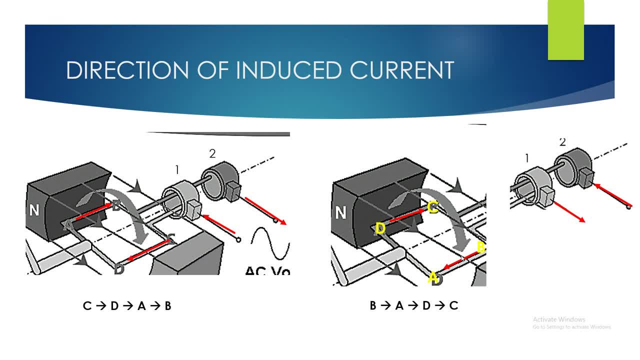 again and see where the current leads you again. the current is still going to be in the direction of current. so you can see that the current is going in this sort of direction, but you can see it's going in the opposite direction than it was before. so it's still going, rotating around. 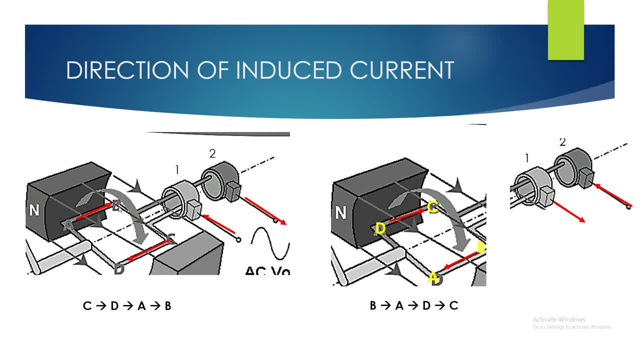 these four quadrants. but remember, if you take a look at this first diagram, the current was going from a to b, and then b to to c, eventually and c to d. but now it's going the opposite. it's going from b to a and d to c. okay, and of course this direction of current will feed into the 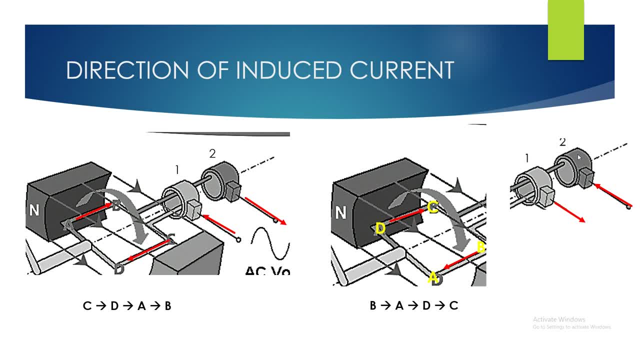 slip rings and the overall current direction will be completely reversed. so every time one side move over to the other side, the induced current will be in the opposite direction. that's why you get alternating current, because each half rotation of the coil you're going to get an opposite direction.